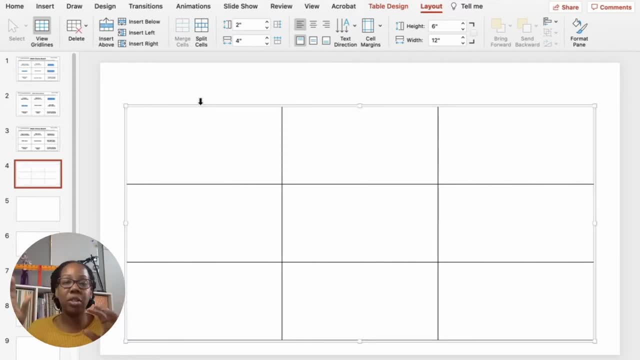 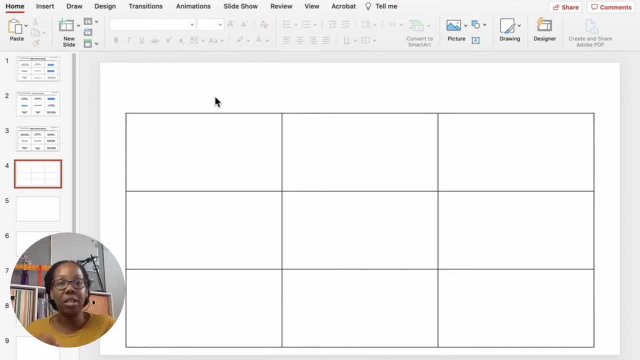 want to add a heading and a place for directions and their name so I can hold students accountable when they have to turn this in. All right, so we have our table. Now we're going to insert our text boxes to show what activities we want students to work on, So I'm going to click into the table. 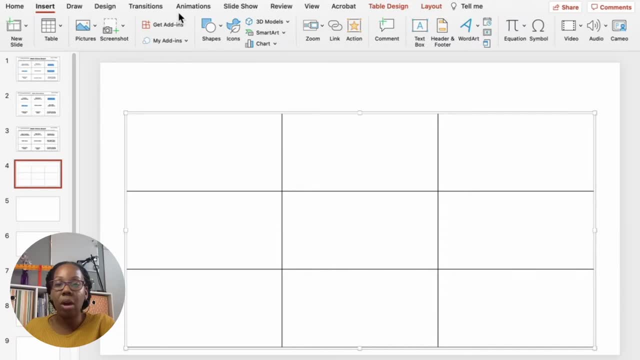 and then go to the insert tab and then go all the way over towards the right until you see text box. Click on that. We're just going to create a text box here and we're going to type out one of the. I'm just going to throw some different options on our choice board to use as examples, So one could. 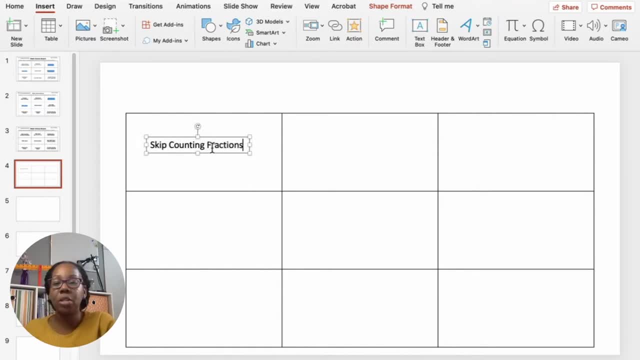 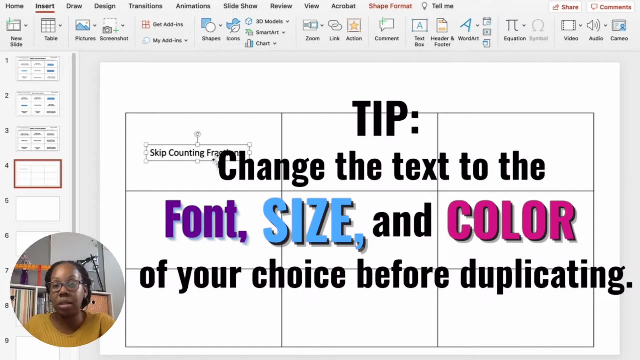 be a skip. counting activity. Okay, so I'm not going to recreate a new text box for each, so I'm actually going to duplicate this text box. Before I do that, I want to change the font, the size, the color, if I want that changed now, before I duplicate each of the text boxes. So I'm going to select. 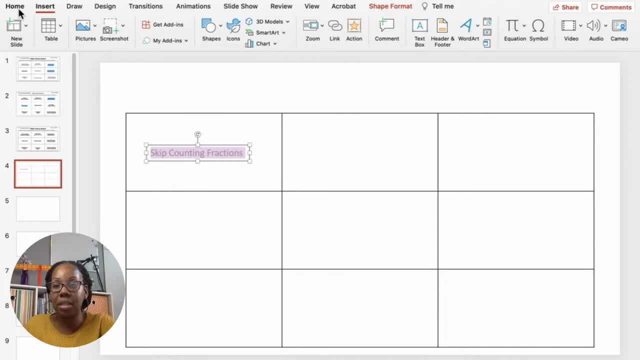 inside of my text box, Go up to the tab and select home. Then I'm going to go over to the font and choose the font that you like the best And I'm going to make mine bold. I'm going to adjust the size. See if that fits. It fits, but it's kind of tight there, so I'm going to go down. 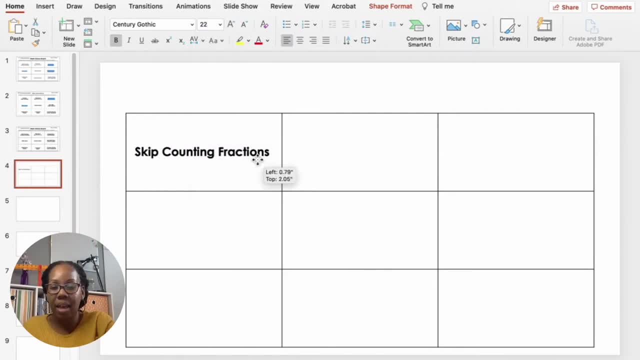 I'm going to type in 22 and that works for me. All right, so we have our first text box in there. So now I'm going to keep that text box selected and I'm going to, on my keyboard, hit command d, or you can hit control d to duplicate. 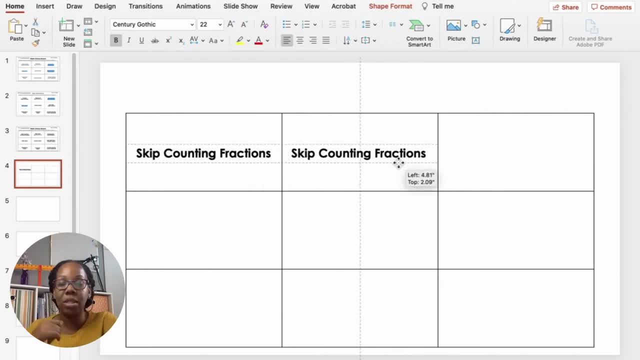 Duplicate that text box and then move it over to the second rectangle or second space and let that go. Make sure it's aligned. If you saw those red lines, it's aligned horizontally and vertically with the middle of the table. So now I'm going to, while it's still selected, hit command d or. 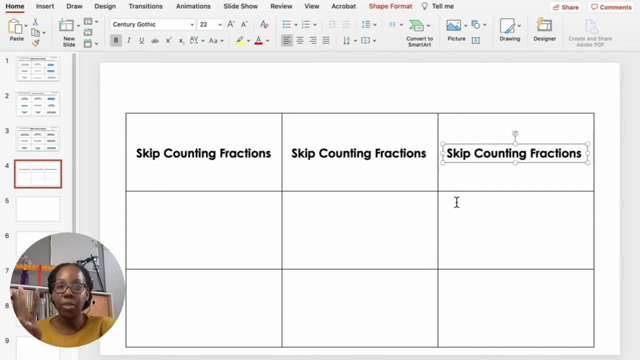 control d again, and that's going to recreate the third text box that I want. Okay, now, instead of duplicating them individually, I'm going to select all the text boxes and duplicate by hitting command d or control d again. And now I'm going to move. 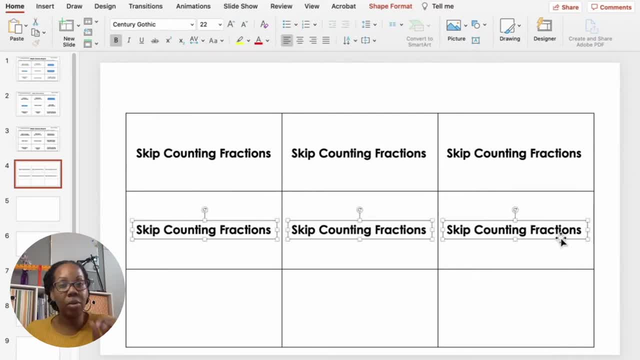 those three down to the middle row. Let go, Keep them selected and then hit command d again, which recreates it on the third row. So now we have all of our text box- not text boxes, we have all of ourselves filled. I'm going to go in and change the wording that I want. So this is where you. 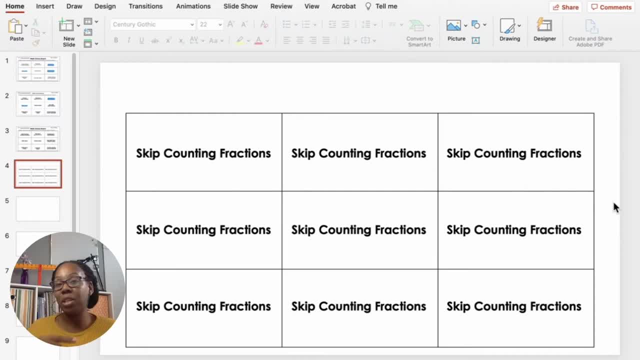 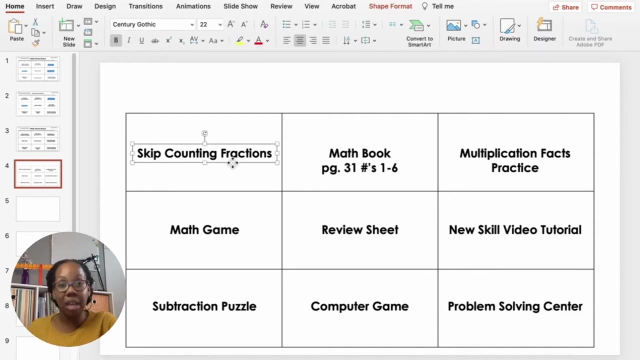 would add in the different activities that you want. So I'm going to fast forward a little bit what wording I change my activities to. All right, so now we have our activity titles in each of ourselves. Now we can add in our header section. So I'm going to take one of these text boxes and 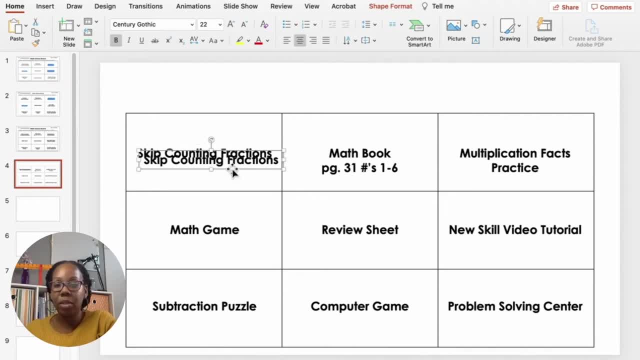 select it and hit command d to duplicate, and I'm going to move it towards the top and change it to name and then change the font if you want to, And I'm going to add and you can do an underscore to it or you can add in a line by going to shapes: Go to insert, insert tab and then go over to shapes. 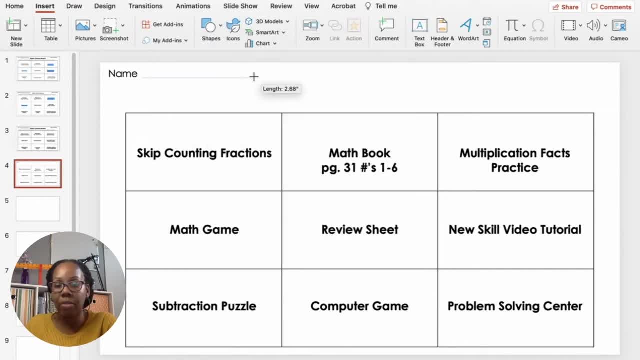 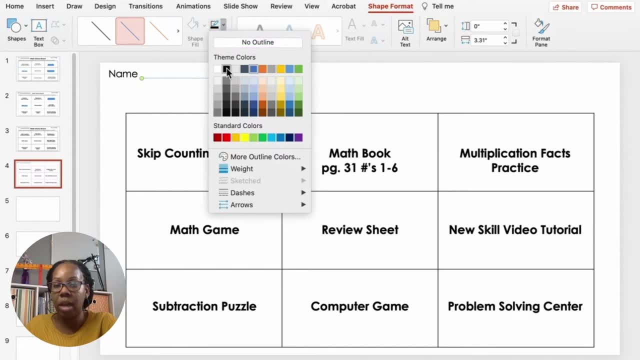 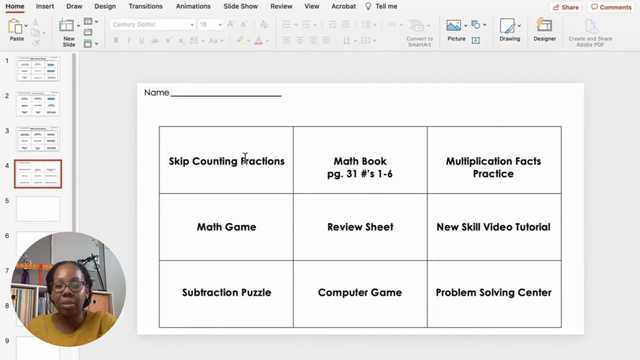 and select line. I'm just going to draw a line there for them to write their name, and then the shape format tab should appear where you can change the color and the weight of your line. Okay, so next we're going to add in our quick heading, So I'm going to take that same text box. 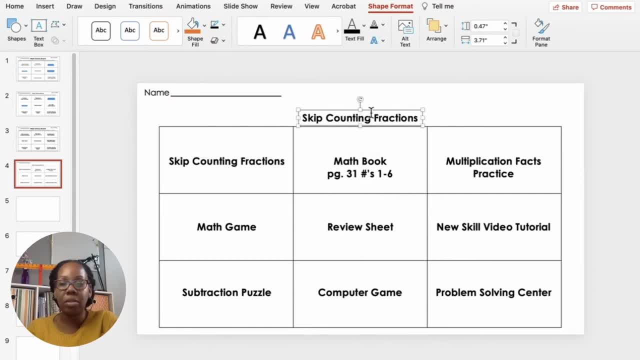 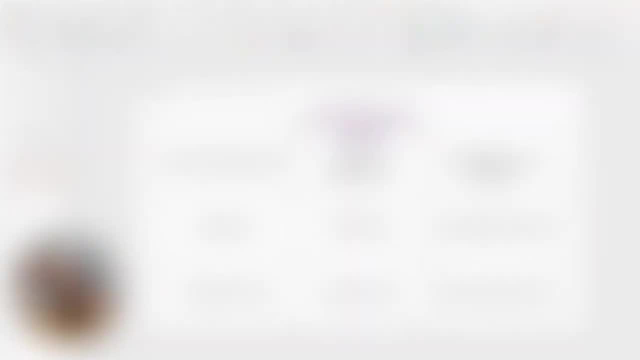 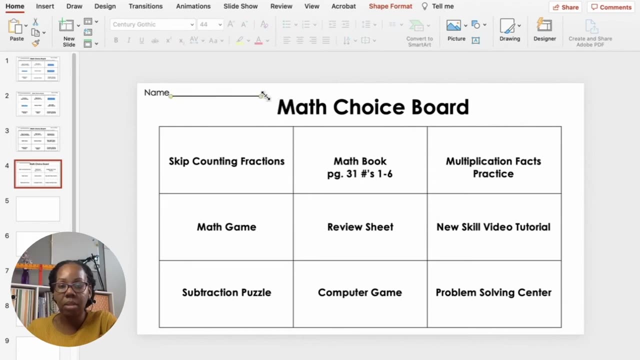 hit command d to duplicate it. Then I'm going to change it to math choice board and change the size. I'm going to keep the same font. All right, let's stretch that out and move that up here. Actually, I'm going to move my line in a bit, so 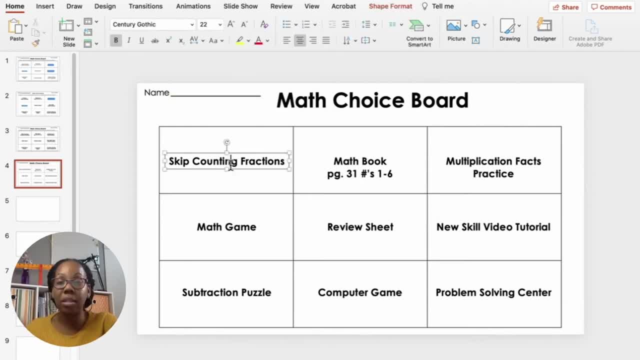 that I can move my title up. So now I want to add in some instructions at the top. So I'm going to hit duplicate for that same text box and move this up here, and then I'm going to type in and want it left the line and stretch out this text box. 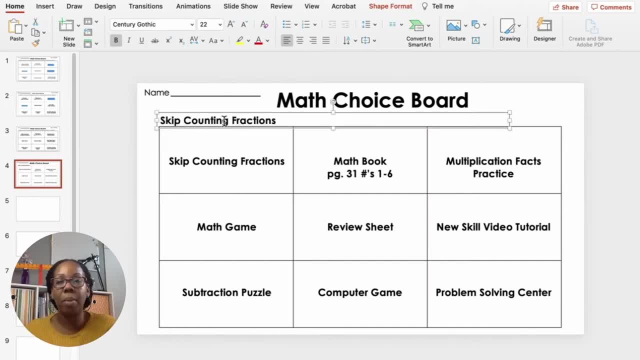 And I'm just going to type in what I want them to know about completing this activity or this choice board correctly. All right, so now I have those instructions for them and I'm going to add a little reminder of when this activity is due. I'm going to leave that up there and bring that down just a little bit. 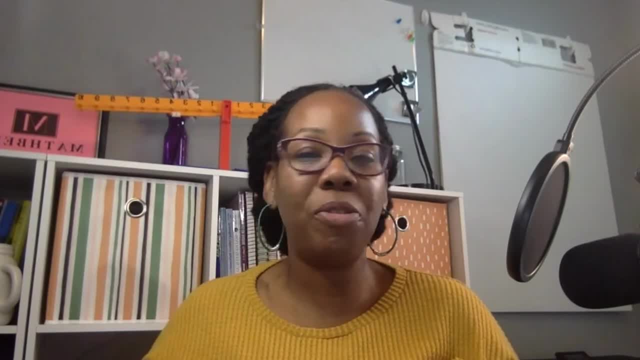 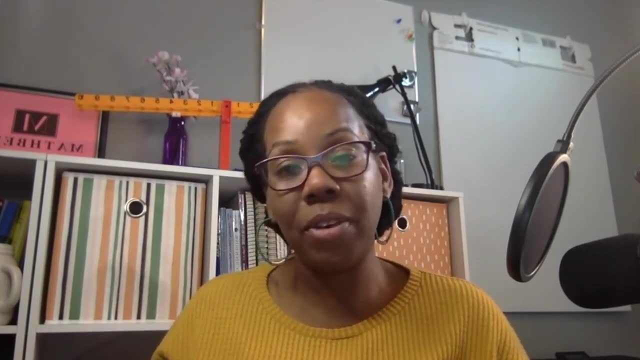 So that's your math choice board that you can create to differentiate activities and tasks for the students in your class. So I'm going to leave that up there and I will add it in here. Let's go class. whether you're working in a classroom and you want to print this out for each student, 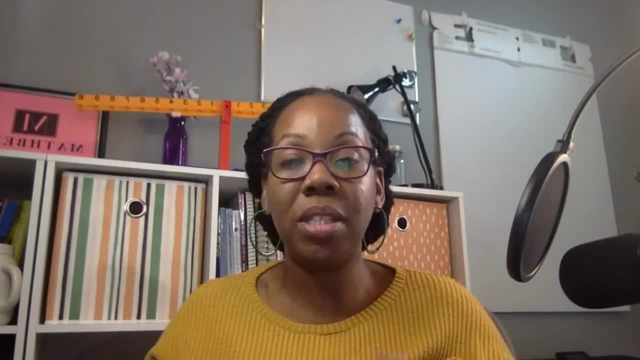 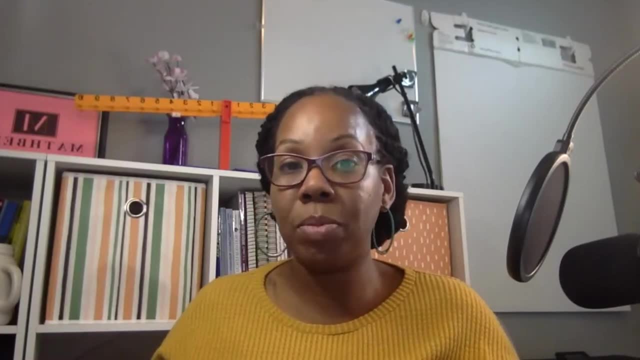 or you teach virtually or in a remote situation where students have access to their assignments online, or even if you're in a classroom and your students have access to a learning management system where you can post activities and tasks for them to complete online. let me show you how to. 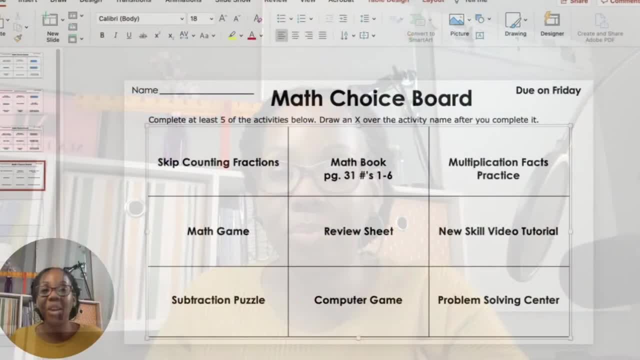 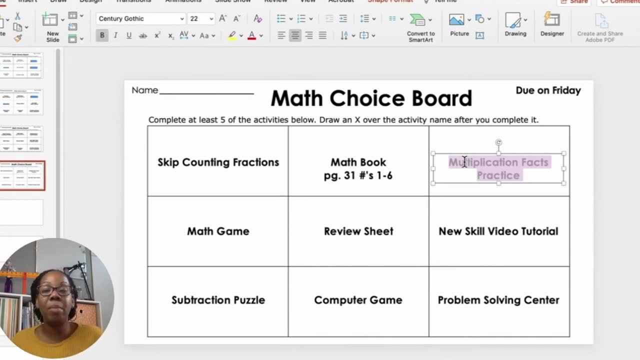 add links to the different activity titles. So if I wanted my students to work on their multiplication facts practice using a specific website or program, I'm going to go to that website and select the link, or copy the link and bring it back, paste it into my text box. So let's. 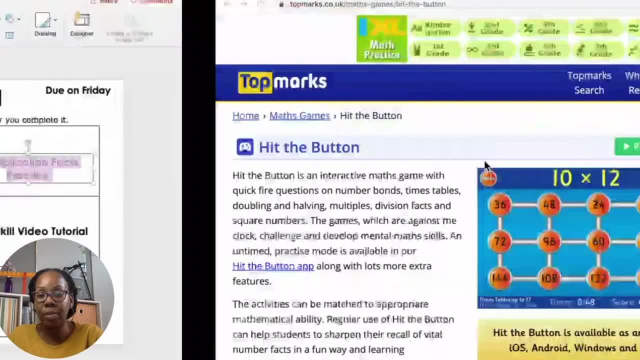 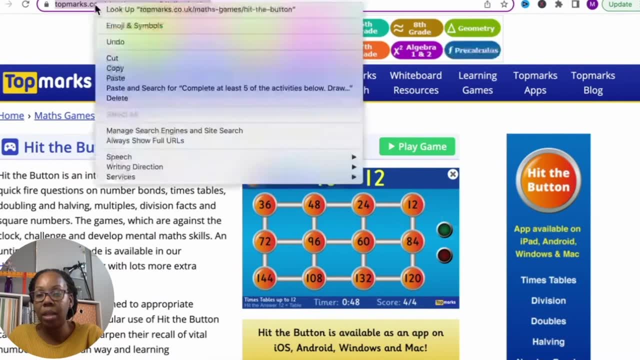 do that. now We're going to go to a separate page, that web page Here. I want them to use the website, hit the button. So I'm going to go up to the address bar, select it and you can right click. 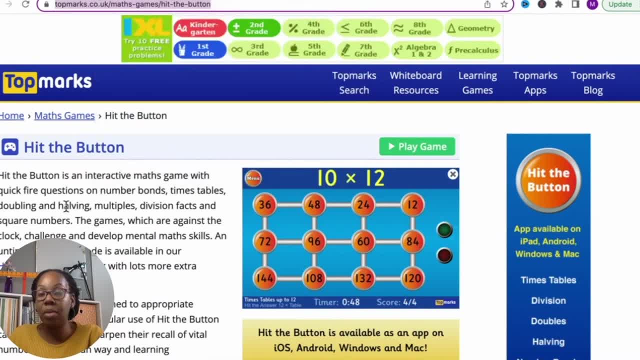 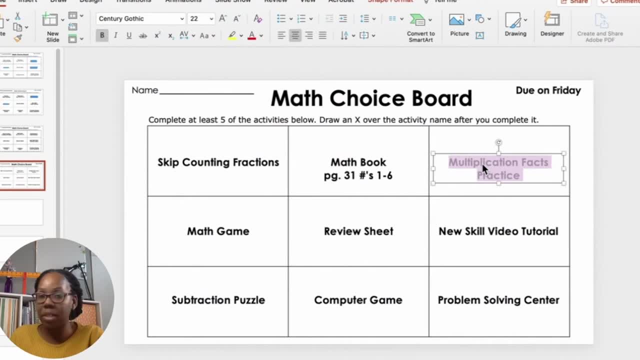 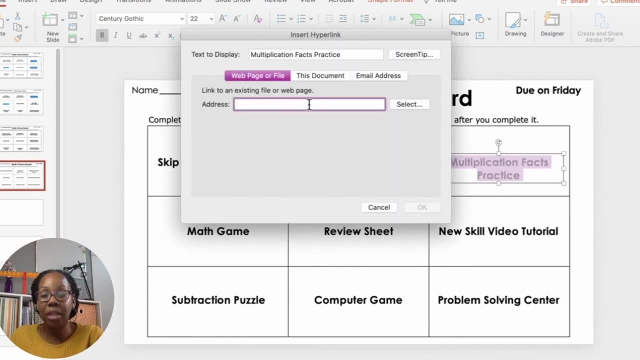 and copy, or you can hit command C or control C on your keyboard. go back to your math choice board while it's selected, or if it's not selected now, and right click and go down to hyperlink insert. hyperlink tab should pop up and where it says address, that's where. 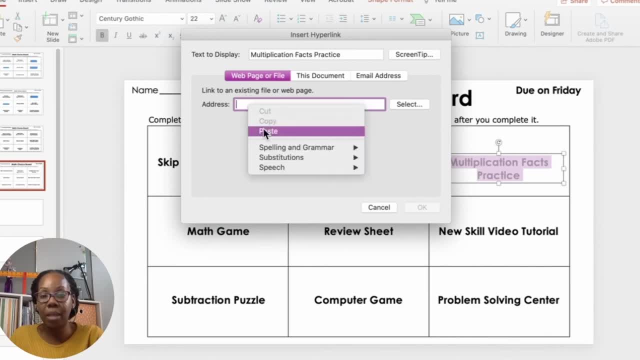 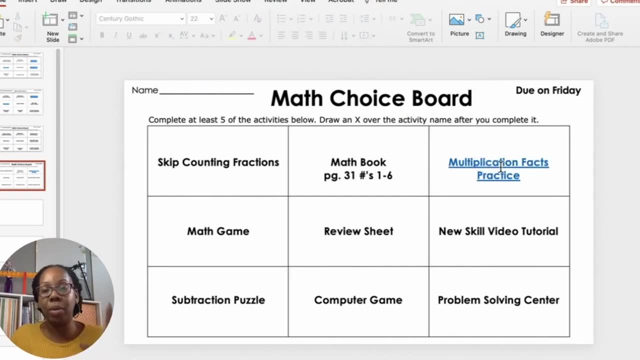 you're going to again right click and paste, Then hit okay and now they can click on that link and it will take them directly to the website that you want them to work on. Let's do another example. But if there's a specific math, 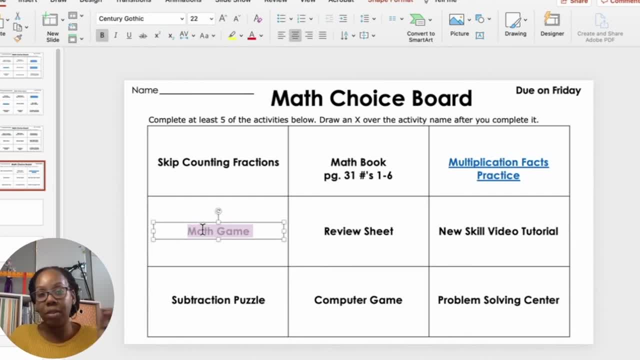 game that you want them to work on, let's do another example. But if there's a specific math game that you want them to work on, let's do another example. But if there's a specific math game that you want them to play on, or for the video tutorial, there's a specific video I want. 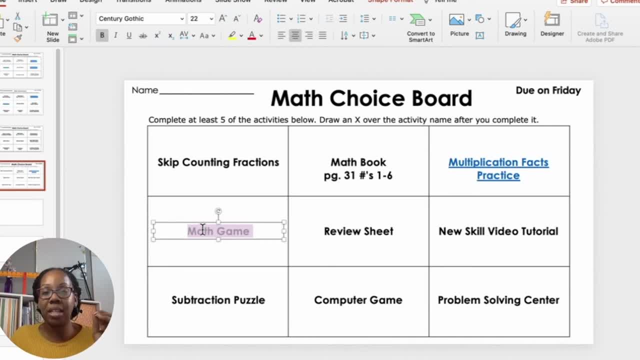 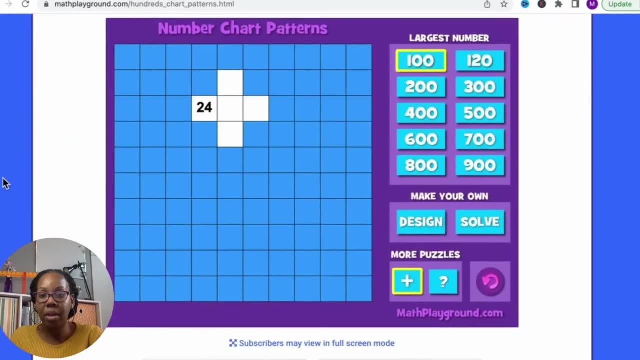 them to watch. I want to copy and select that specific web address so that when they click on the link through my math choice board, they go directly to that page. So let's go to our math game that we might want them to play. I have a game here where they're